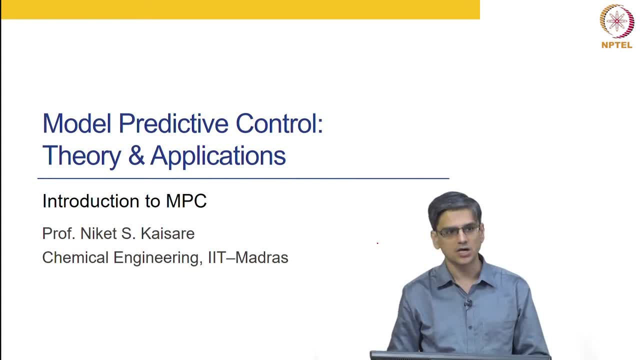 we are kind of going to cover them all All over again, but the focus is going to be on vectors and vector spaces and linear transformations and so on. So it is kind of concepts that you are familiar with but unless you have taken linear operators type of a course and an advanced linear algebra. 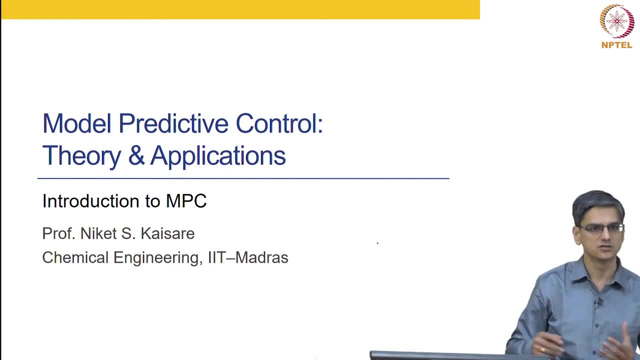 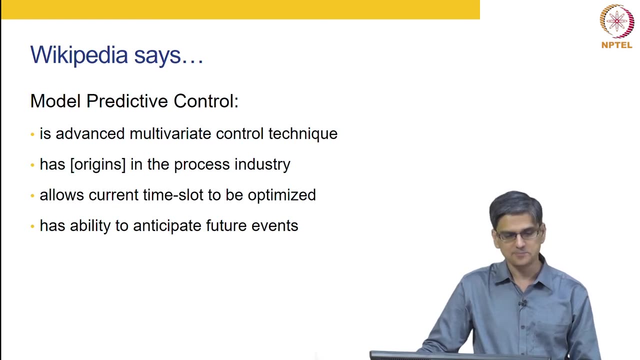 course, this would be a little bit a new flavor to doing the same things. ok, But today, though, we will talk about introduction to MPC, And this is just the information about MPC from Wikipedia. So MPC is a advanced process control approach or advanced multivariable, variate, multivariate control technique. It 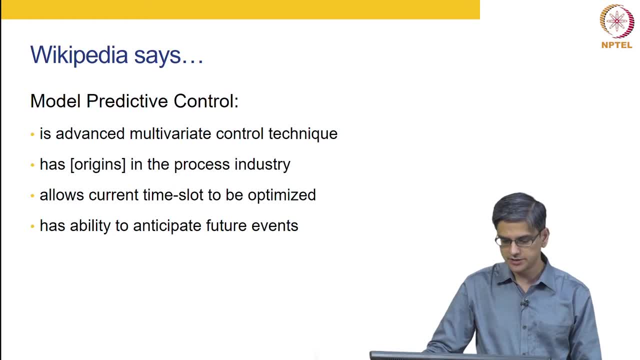 started in process industry. as I have said multiple times, The important part about this, it is an optimization based algorithm, So it allows current time slot to be optimized. We do that in ah, what is called as a receding horizon manner. Ah, we use a model to predict. 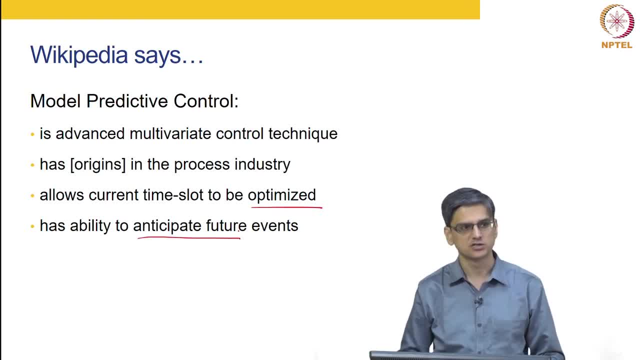 the future. So that is why it says anticipate future events: ah, Something that we will come to in probably week 12, the last week of this course is: ah, this anticipate future events is about 2 things Pretty much for 10 or 11 weeks of the course. we will talk about what. 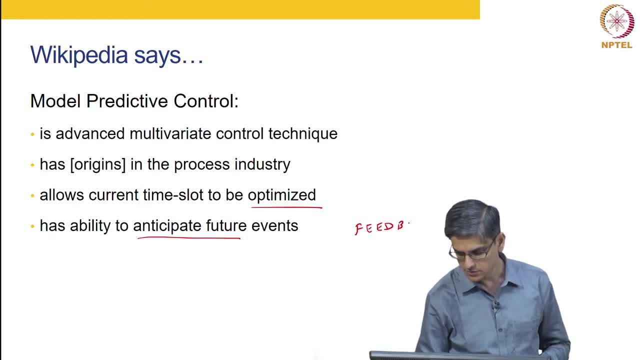 we call feedback, feedback, Feedback, Feedback, Feedback, Feedback, Feedback, correction. ok, What that basically means is that you measure, ah, you take a few measurements, and then you correct: ah, because there are going to be errors in the models. there are. 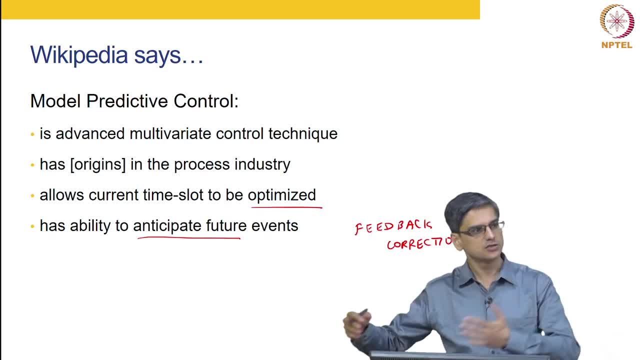 going to be certain uncertainties, you correct for those errors and then you keep doing that. ah, all over again. ok, So that is ah, one approach and that is the standard approach. Ah, The other approach, or the more, ah, more advanced approach, if you can, if you can call. 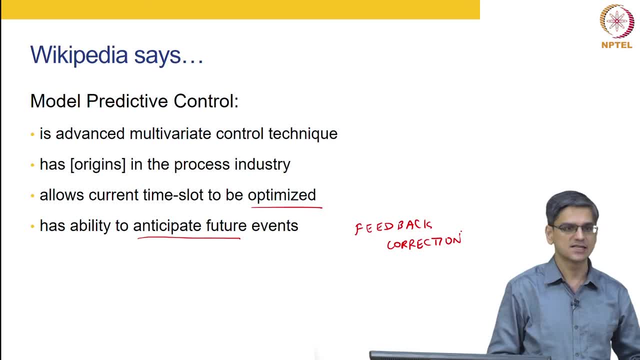 it, that is, to quantify these uncertainties, and can you use the past in order to predict also how the uncertainties are going to behave? And that is ah, basically one more ah, one more aspect of ah, of MPC. ah, ok, The former aspect is ah. MPC is said to be optimal in open loop. 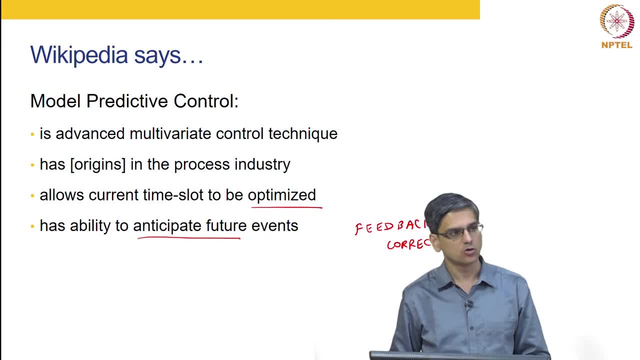 sense. in the latter aspect, the MPC is said to be ah, optimal in closed loop sense. For most of you in this room, probably the last ah statement would not be there. It would not have made sense. ah, hopefully by end of this course it will make a little. 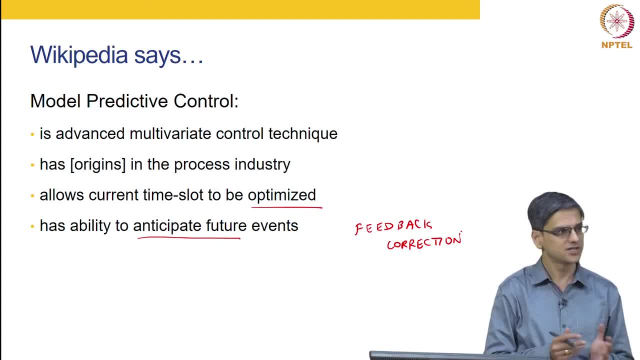 bit more sense. Ah, There are some PhD students over here for you guys may be, you may know the distinction between something that is open loop optimal versus closed loop optimal. Ah, But again, this is something that hopefully, by the end of this course, we will get an idea. 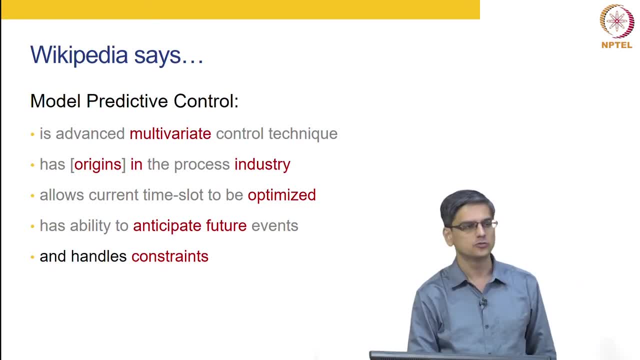 of ok. Ah, From my point of view, one of the biggest reasons for MPC success in process industry is- Or are these two things multivariate and ability to handle constraints? ok, This is again something that I said last week. ah, just this is just reiterating that. Ah, Initiated in shell oil. 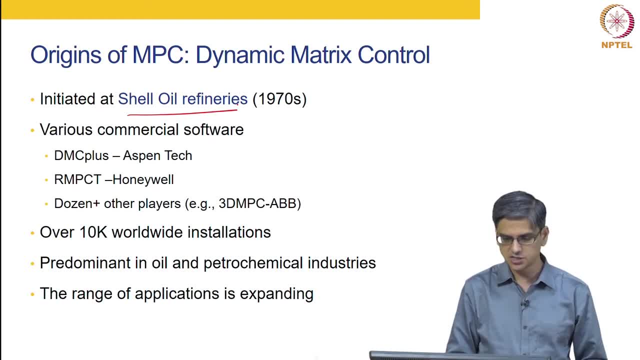 refineries, ok, And the first application of ah MPC was called DMC. DMC stands for dynamic- oh, ok, we have this over here. ah stands for dynamic matrix controller. ok, Ah, ah. ah, this that was. it was a company called DMC. ah, the DMC company was bought over by Aspen Tech. 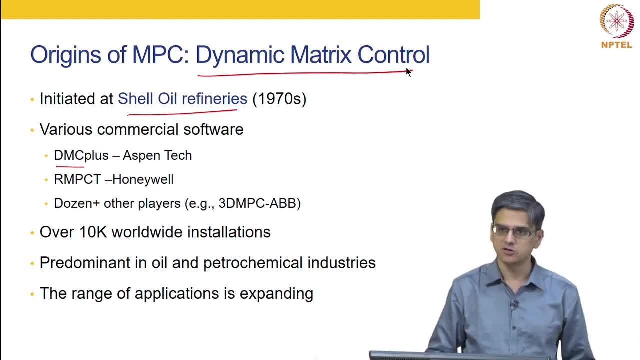 and even today, ah, a variant of the DMC algorithm is available, ah, in the industry, Ah, And then there were a lot of players, almost ah, you know 10 to 15 ah automation providers ah, started providing MPC, ah, ah, and so it is. it has commercial origins, ok, It is predominant in oil and petrochemical. 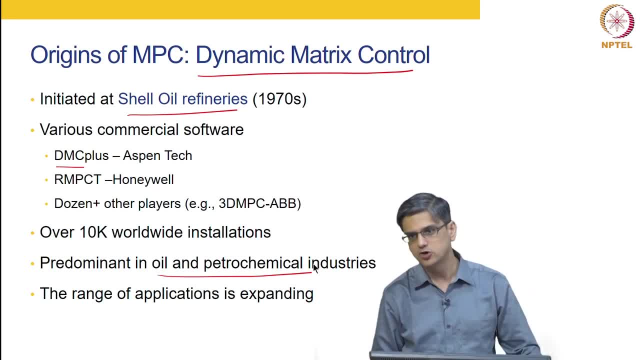 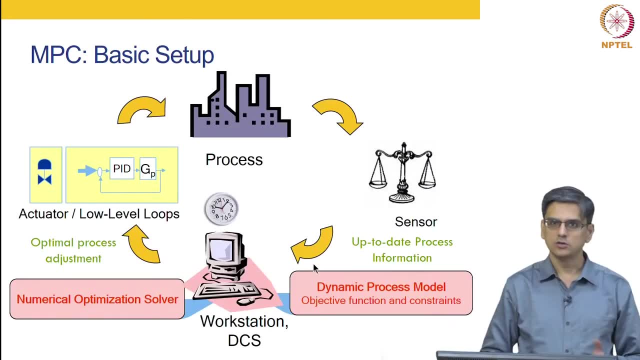 industries, and that is now changing, ah, it is becoming more and more popular in ah, electro, electrical and mechanical and electromechanical systems and maybe even aerospace system. ok, So let us talk about the basic set up for MPC. So we have this process over here, ok, Ah. And then there are sensors and we talked ah. 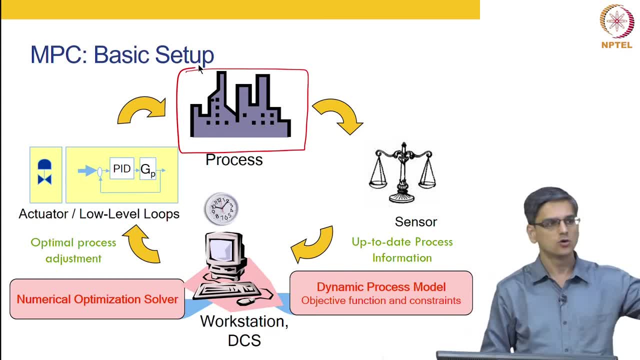 in the previous lecture that sensors are going to measure only some items that are important, ah to us for controlling a system. ok, So sensors do the measurements. ok, From the measurements, we use an observer in order to get the state information. ok, There is a dynamic process. 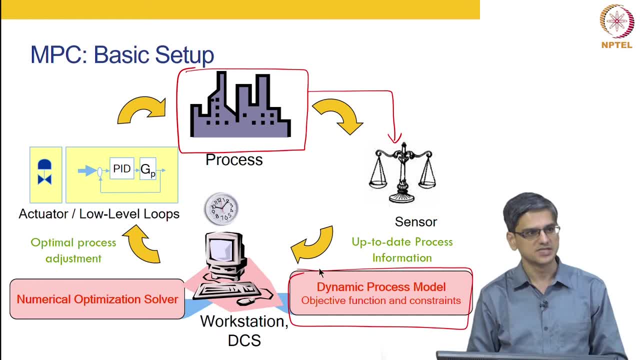 model that is present in an MPC algorithm. The process model is used to predict the future. ok, The process model runs in some kind of a computer, So it could either run in a centralized computer or it can run in a decentralized manner in a DCS system. ok, 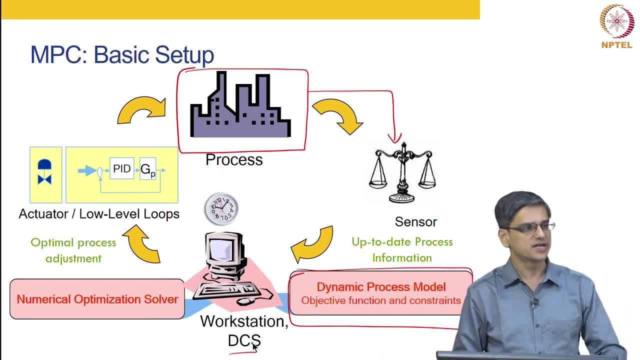 What is done in MPC is we predict how the future is going to behave for various different sets of input moves and then an optimization algorithm selects the best set of input moves in the future. ok, So let us say we are at time 10, we will predict the future at time. 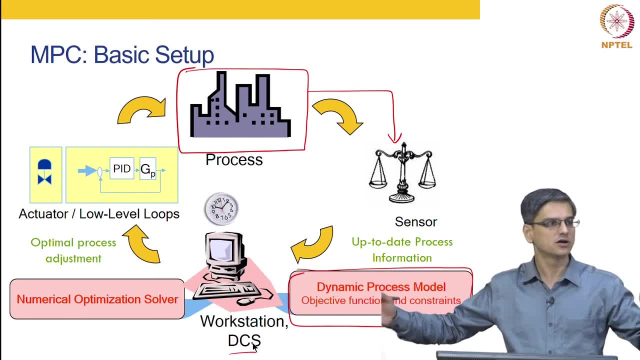 11,, 12,, 13,, 14,, 15. that was make a prediction horizon of 5 steps into the future. We will optimize and determine what is going to be the inputs for the next M number of steps. ok, But we are not going to implement all those inputs. we can only implement a. 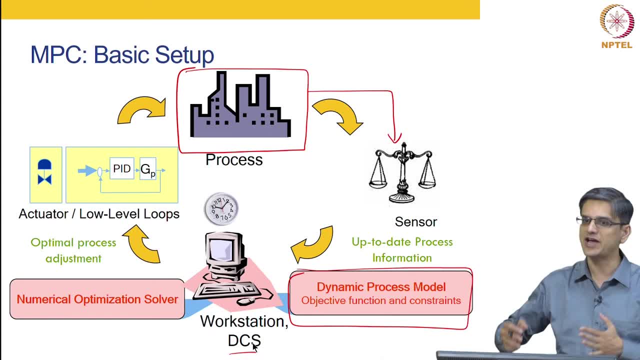 current input, So at time 10,. although we have calculated inputs at time 10,, 11 and 12,, we will only go ahead and implement the input calculated at this time That is sent as some kind of a set point to a lower range. So that is what we are going to do here. 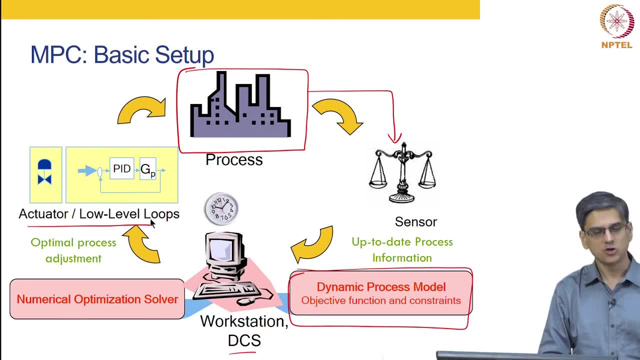 Cover further. we talked about hierarchy of process control, right, and that lower level control rule determines the flow rates, for example. or you know, the final contact element, how that finally control element is going to move in order to meet this particular requirement. ok, And that is done all over again. time 11, at time 11. prediction is from 12,, 13,, 14,. 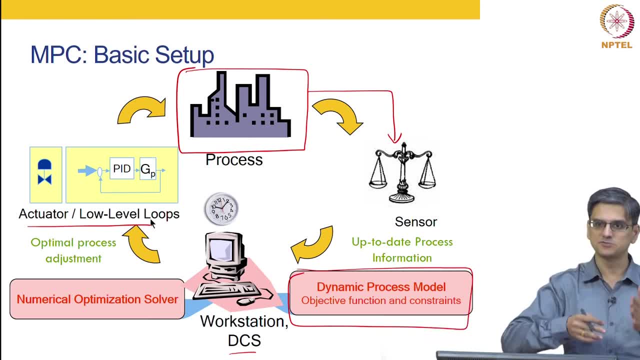 15, 16,, at time, 12. prediction is from: 1.不 Prada, 19.不产来0.. MN gate. It is very from 13,, 14,, 15,, 16,, 17,. okay, You would have noticed, when I talked about 10,, I said 11 to 15,, when I talked about 11,. 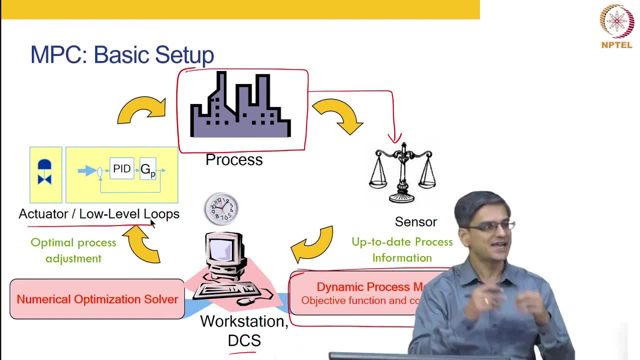 I said 12 to 16, why? Because 10 has already happened. You cannot change anything about 10.. So there is no prediction about 10, it is just how the system has responded at 10, prediction is from next time steps into the future. okay. 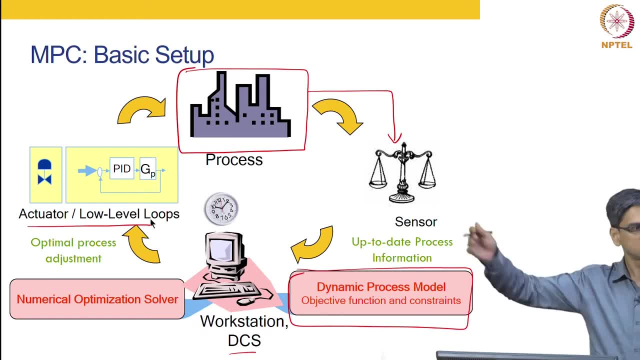 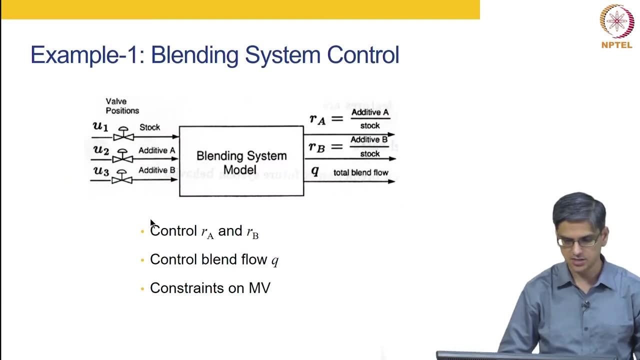 And, if you have noticed, I said 11 to 15,, 12 to 16,, 13 to 17.. So that is a horizon and that horizon keeps moving. okay, and that is called a receding horizon, implementation. Again, these are the terms that I talked about in last week's class. 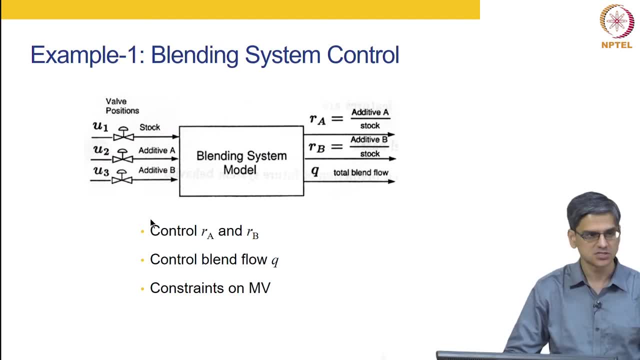 Let us again look back at the example of a blending control system. okay, Let us say that we are interested in controlling these two variables at the desired set point. okay, We want to control q. We want to control q also at their desired set point. 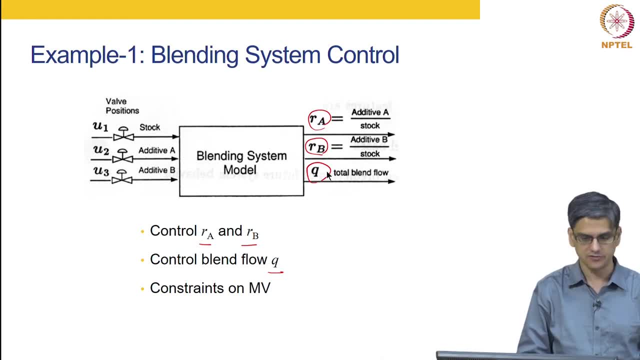 In addition to that, there are certain constraints on manipulated variable. For example, the u1, u2, u3 should be greater than 0 or may be greater than equal to. This is a very good question. So the question is: let us say we are currently at time 10, okay. 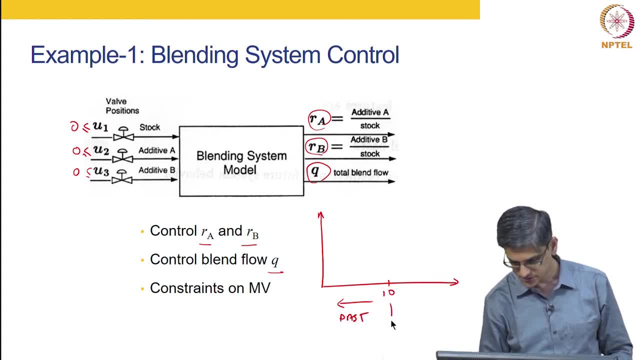 This is past, This is present And this is future. okay, Let us say we have somehow reached over here. The question is: does the past trajectory matter? okay, The answer to that question is yes, the past trajectory matters. The other question, which was specifically what the question he asked, is: do we need? 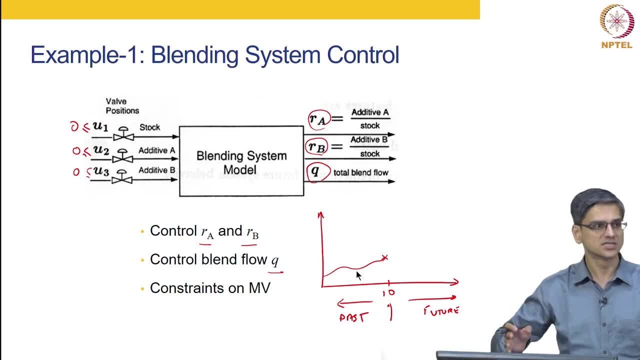 to keep in our memory all the past, That is, 0,, 1,, 2,, 3,, 4, up to 9,. do we need to keep in the memory? The answer to that question typically- usually- is no. 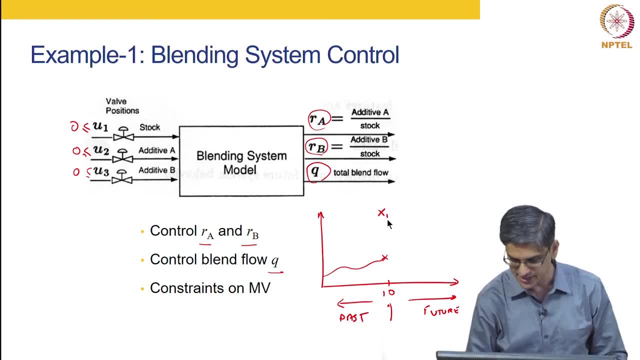 Why? Because we have defined our state, x k, as something that has all the information that is present in order to predict the future. okay, So x k somehow is capable of carrying the information of the trajectory. Okay, So x k is the data. 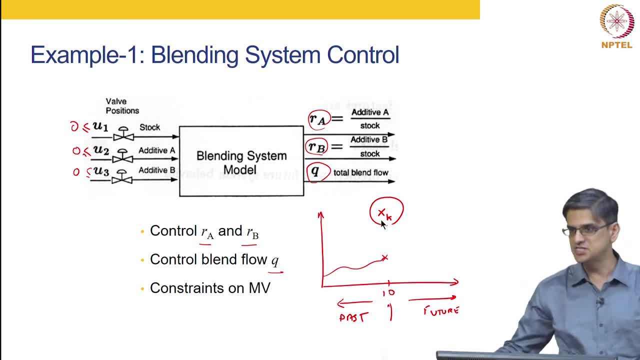 So x k is the data. So x k is the data. Okay, So x k is the data of the trajectory with respect to predicting the future behavior using the model. okay, It does not have all the possible information about the system. no, 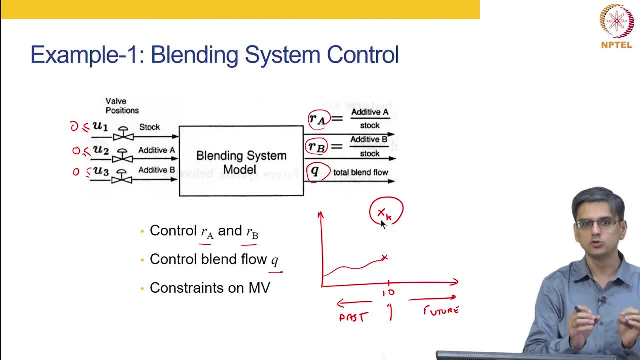 It has all the information that is relevant for you to use the model in order to predict the future. That is the assumption that we are going to use. okay, So under that assumption, the information that you need is x 10 in order to predict. 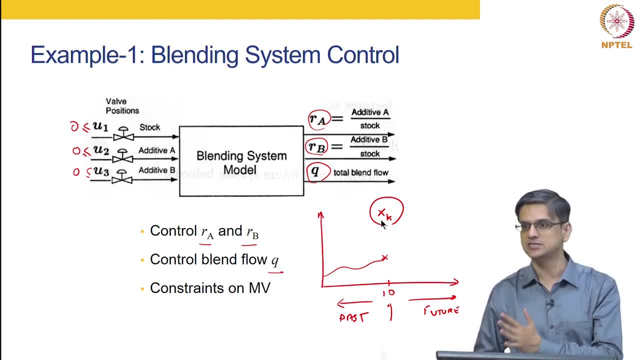 the future. okay, In next week's class We will actually take, We will actually take up a. take up an example what that means. There are examples of finite input, finite impulse response models, where you keep certain information of the past in your memory. 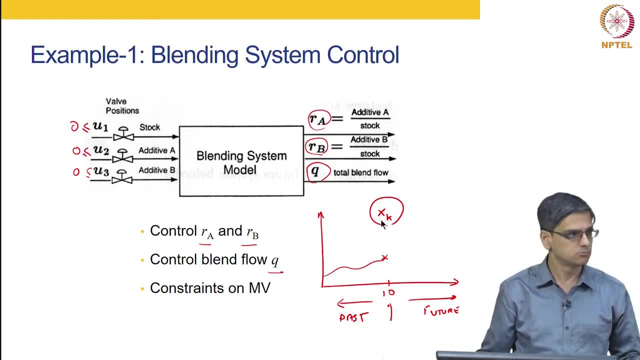 Then there are something called ARMA model. So people who have done or are doing time series analysis course might have come across these models where you say that in order to predict future, I need to keep information, I need to have 4 time steps in the past or 3 time steps in the past. okay, 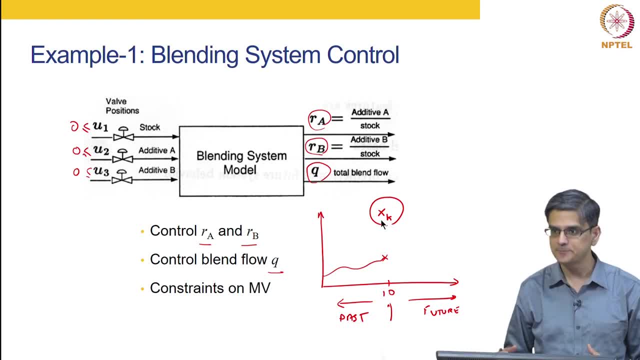 So, yes, information of past is required, but we define states such that x 10 is sufficient to predict x 11,, x 12,, x 13,. okay, So the shorter answer to this question is: x 10 is sufficient. sorry, 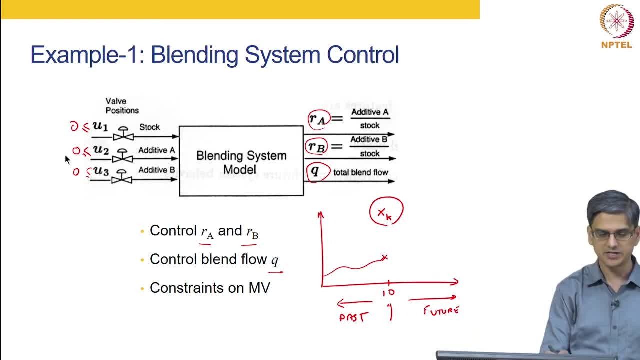 Yeah, And yeah, there are constraints on manipulated variables and there could be constraints that we want to meet on these variables as well. Okay, Yeah, So it is not just the constraints on manipulated variables, but there could be constraints on controlled variables as well. ok, 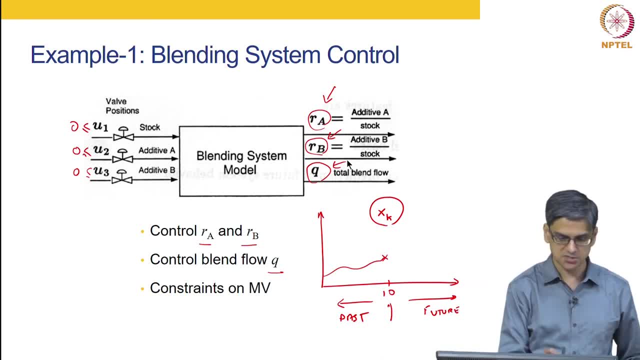 The traditional approaches for APC can handle constraints on manipulated variables. lot of times they find it difficult to handle constraints on ah controlled variables. Not so with MPC. MPC does. it does not matter where the constraints are ah structurally it is capable of handling. 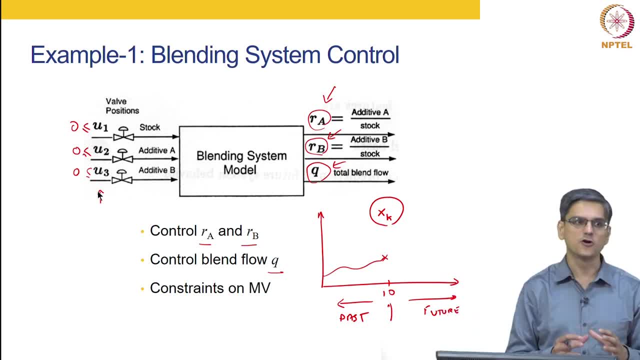 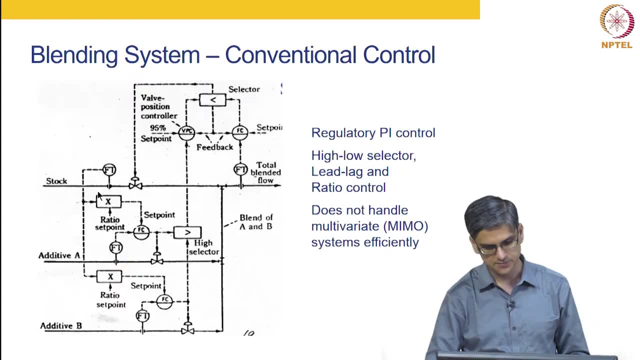 It is possible that certain ah problem formulations are such that it is not possible to handle it. but in general, as a structure, yes, it is possible to handle it in MPC. ok, ah, So the conventional control system uses regulatory PI controller, several other controls. 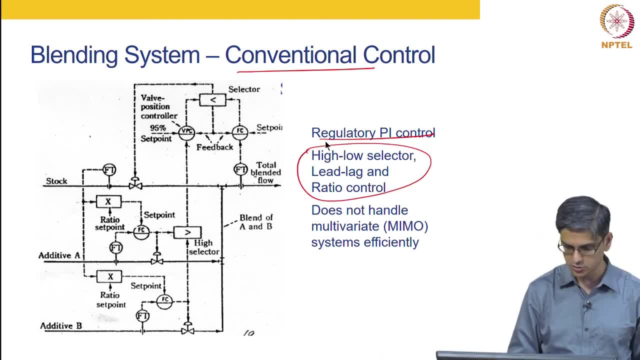 such as high, low selectors, lead lag, type of control, ratio control, and so on. So, for example, this is a ratio controller, ok- which basically looks at the ratios and then determines how. what is the ratio? What is going to be? ah, the set point. 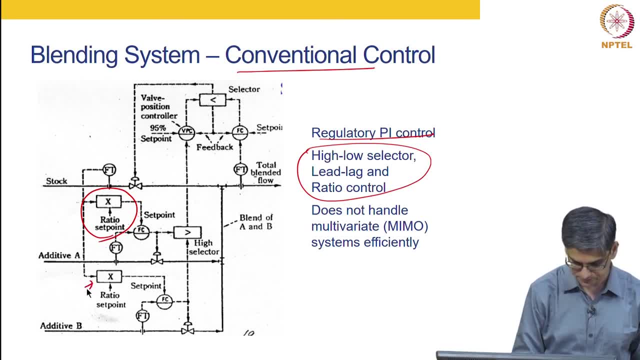 So it takes this value, ah, ah, sorry, it takes this value. it takes this value, ok. uses the ratio in order to determine what is going to be the set point, ok, ah. So conventional system is basically composed of multiple CISO loops that are handled together. 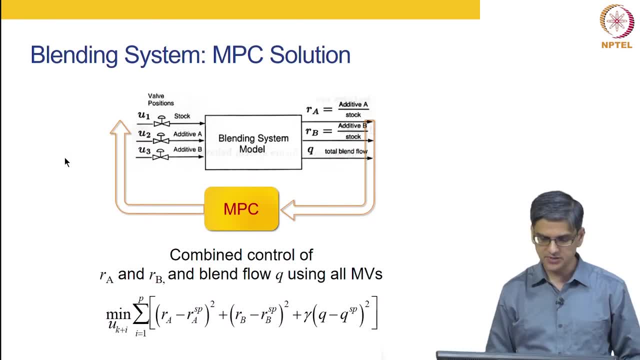 ok. As against, the MPC solution is multiple output, multiple input system, So the set point system is handled as such. it is handled in a multivariate way. ok, and the optimization problem is posed in this particular form, which means your R a is to: 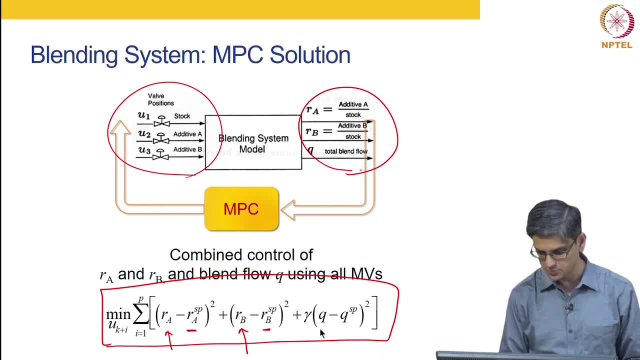 be kept at its set point. your R b is to be kept as a set point. your Q is to be kept as a set point. ok, and these gammas, there would be gamma a, gamma 1, gamma 2, gamma 3, ah, but 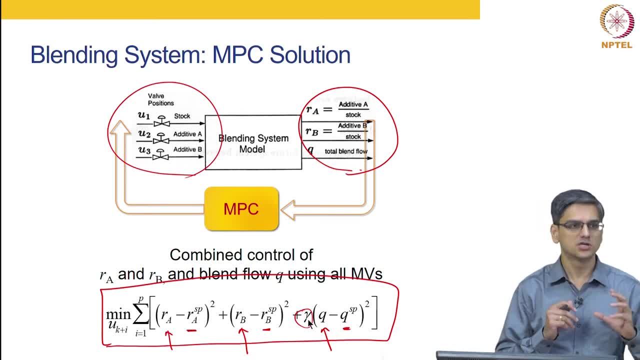 in general. these gammas. Gammas are used to tell the algorithm: what importance do you give to R a, R b and Q in relative terms? ok, It is also used, for example. let us say: ah, R a is in the range 0 to 1, R b is in the. 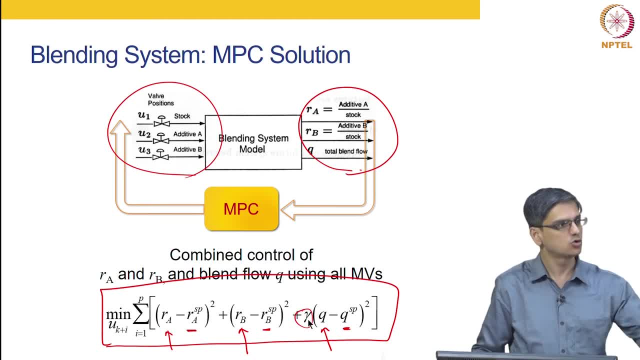 range 0 to 1 and Q is in the range ah 0 to 100. ok, Then we may want to use gamma as 0.01 squared, So that all three are weighed in the same area. Ok, In the same order, ah. in the same order of magnitude: ok. 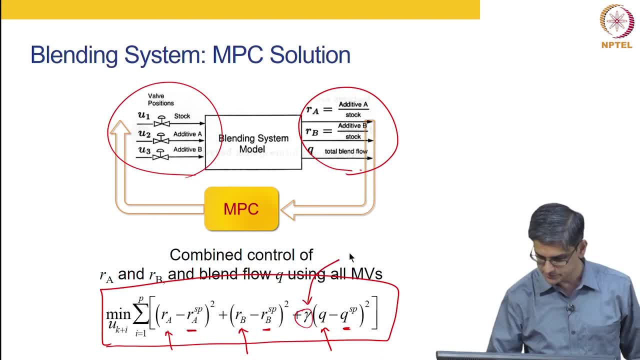 So this is known as weight. ok, and this entire box is an objective function. ok, and we will talk about this when we come to MPC bit later. ok, So, as you can see, it is one objective. So somehow you are trying to say that we want to minimize some kind of a weighted sum. 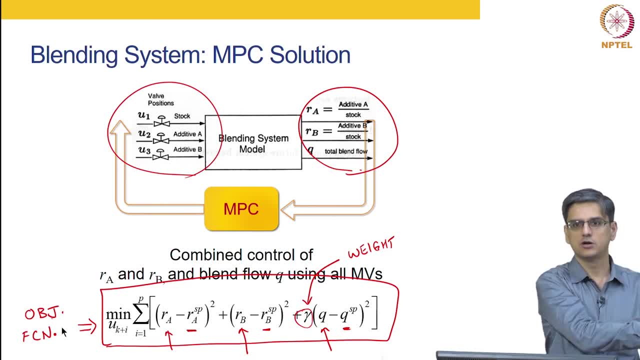 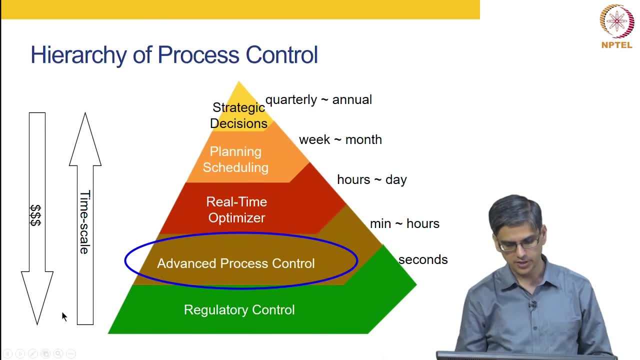 of ah: deviation from set point of ah variable 1 and variable 2 and variable 3, R, a, R, b and Q. ok, and where does ah MPC sit in this overall hierarchy? It sits at the ah advanced process control layer. ok, and that is what I meant when we 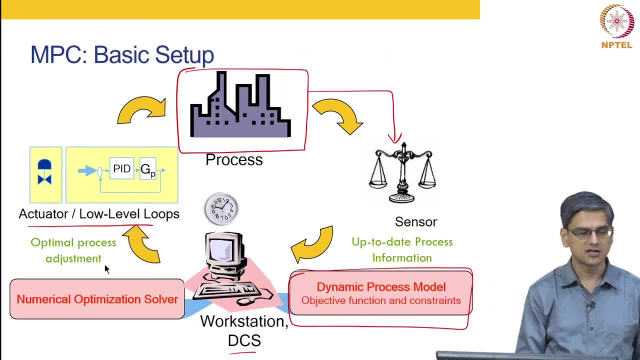 said over here is MPC. Ok, Ok, Ok, Ok, Ok, So MPC determines what ah the set points are going to be for the lower level loops. ok, There are very few instances where MPC directly ah implements those set point. on the final: 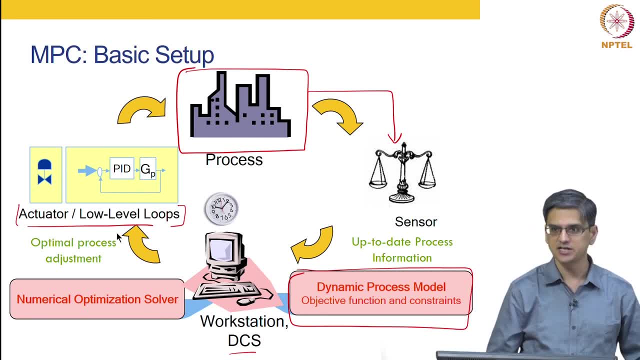 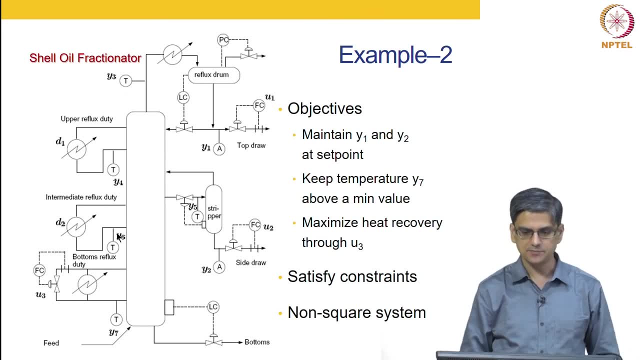 control element. It is usually going to be a PI or PID control that implements the final control element. ok, Another example. ah, this is an example, or a kind of simplified form of this. example is something that We will do for your first project, ok, 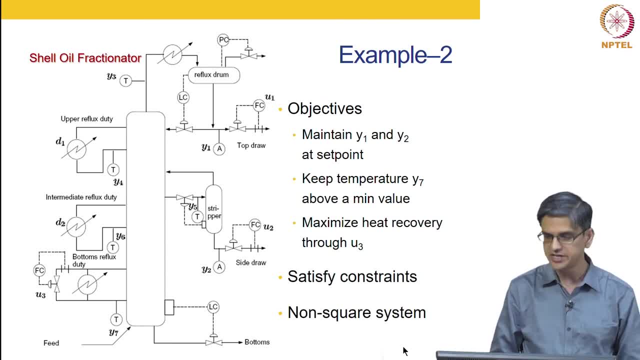 This is a 7 output, 3 input system: u 1, u 2, u 3,, 3 input and u 1 to u 7. y 1 to y 7 are going to be, ah, the 7 outputs. ok, and the objectives is going to be to maintain the quality of. 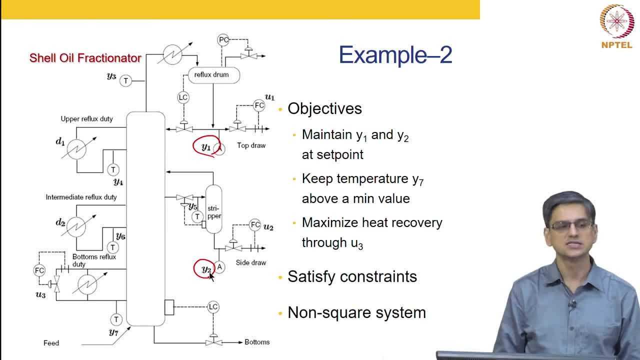 top draw and a quality of side draw at its desired set point. So this is a fractionator which basically- ah, you know, at top draw- We have talked about an ethylene plant or a propylene plant, ok, Fractionator is one of the devices that is used in a similar plant, like this: 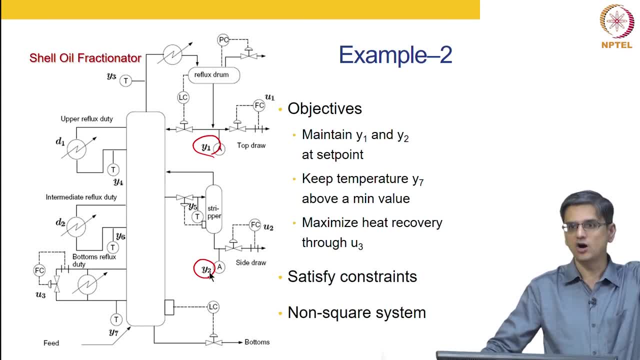 So your set points is that the quality of the most volatile compound and the quality of your middle volatile compound are kept at the desired set points. In addition to that, the temperature of the bottoms has to be kept above a particular value. ok, ah, and you want to minimize? 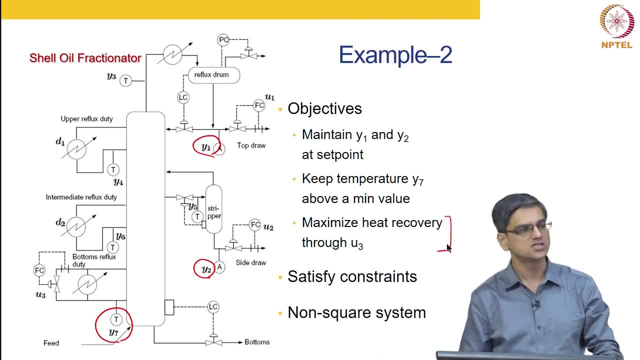 The heat recovery through u u 3.. So these are all conflicting objectives. So there are objectives of keeping things at set points. there are objectives of maintaining certain ah constraints. So this is an example of an output constraint: y 7 has to be kept above a certain value of. 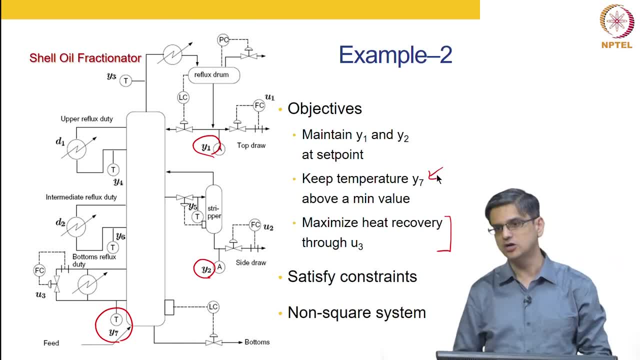 temperature. ok, This is something that is not very easy to handle, ah, using conventional control techniques, but MPC, as we will see, As you will, as you will solve as part of project one, ah, this is something that MPC does not, ah it, it poses challenge to MPC, but structurally, MPC is competent to handle this problem. yeah. 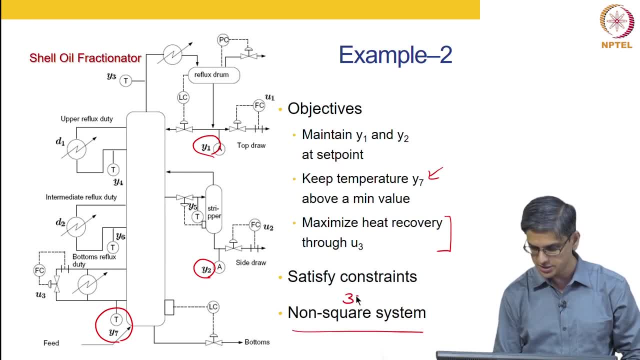 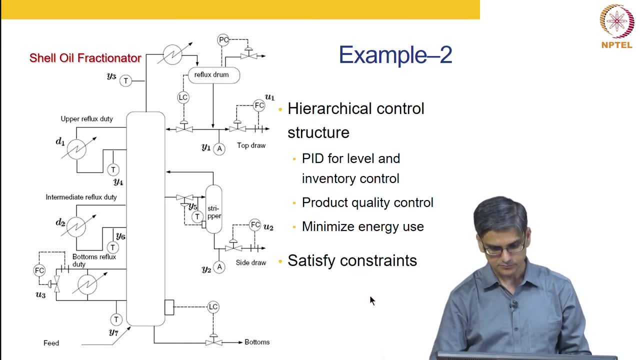 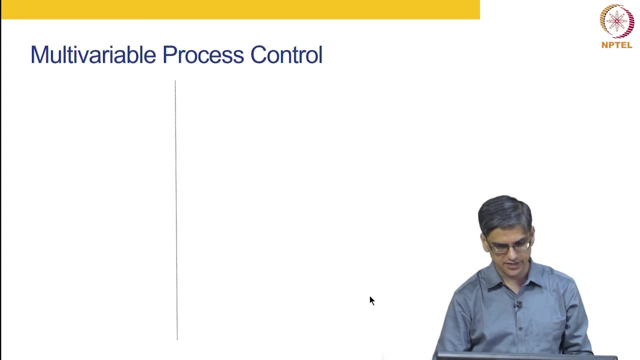 and yes, the other thing is non-square system. right, it is 3 input, 7 output system. Number of inputs and number of outputs are not equal. ok, And this is the example that we talked about In ah week 0 while motivating the ah system. so let us look at the multivariate process. 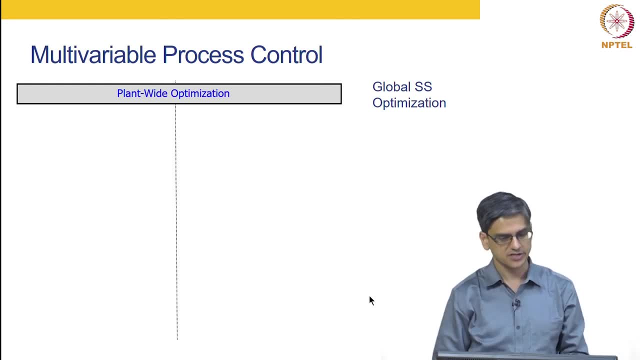 control. ah, the various hierarchy that are present in multivariate process control. The first, the top most hierarchy when it comes to multivariate control systems, is the plant wide optimization. ok, Usually it is a steady state optimization which determines how an overall plant is going to be run. 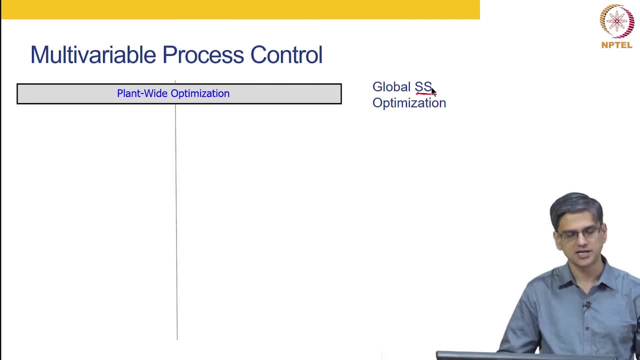 But these days people have been talking about dynamic optimization. So we are talking about dynamic optimization. Ok, We are talking about dynamic optimization carried out in ah. this layer also Plant wide optimization. it is also called RTO- real time optimization. Now, that corresponds to ah individual unit level, local optimization. 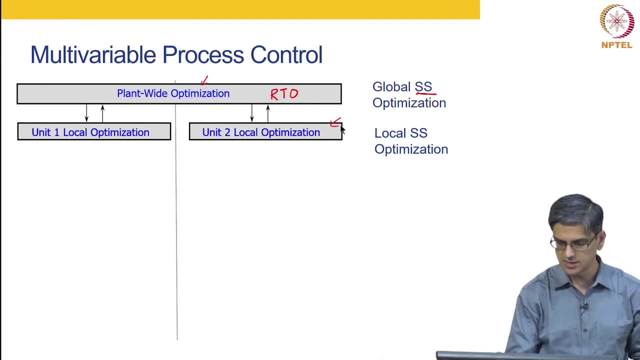 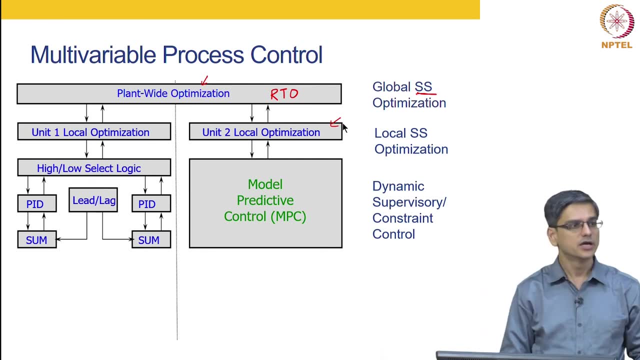 So this is at the plant wide plant level and this is at individual unit or individual subsection level. ok, In traditional control you have you had ratio control or high, low select logic, Lead lag and all of those things sitting in the APC layer. ok, 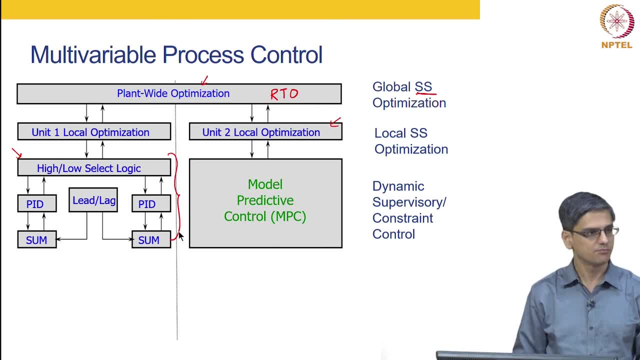 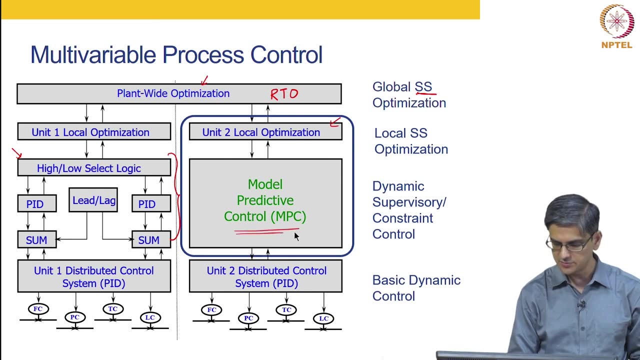 This entire complicated structure is replaced by MPC. ok, What this magic is, what this black box of MPC is, is something that we are going to learn. ok, And finally, the- the decisions that are determined by the MPC layer are passed on to individual. 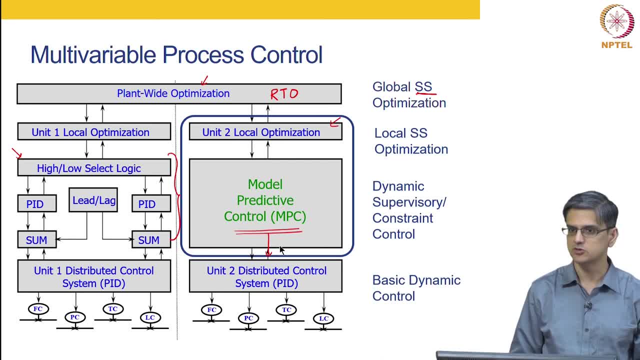 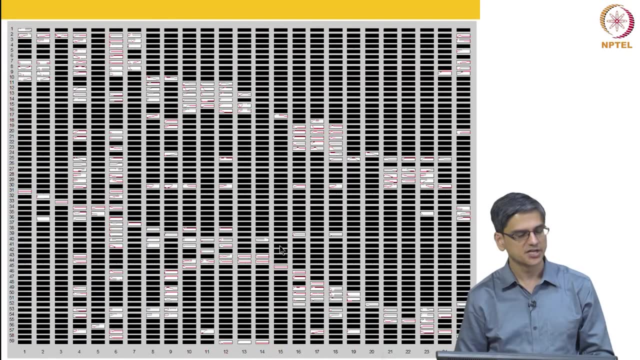 control elements, that this is, ah, something that I have talked about, ah, couple of times already today. ok, And it is these individual control elements that are going to implement the final control action. ok, And this is an example of a typical scale of MPC. ok,